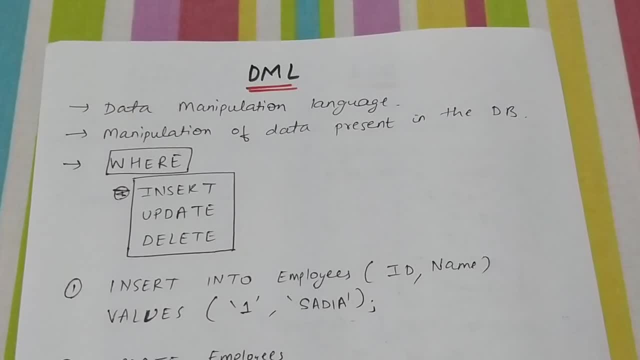 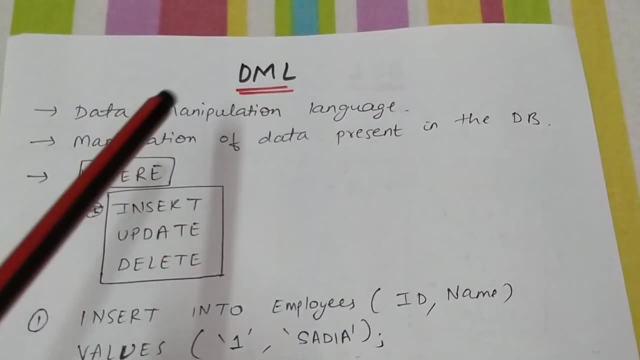 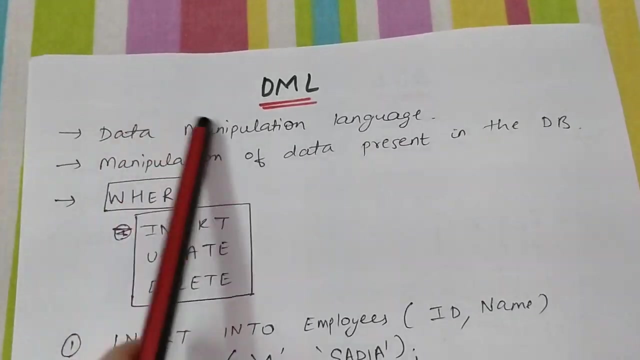 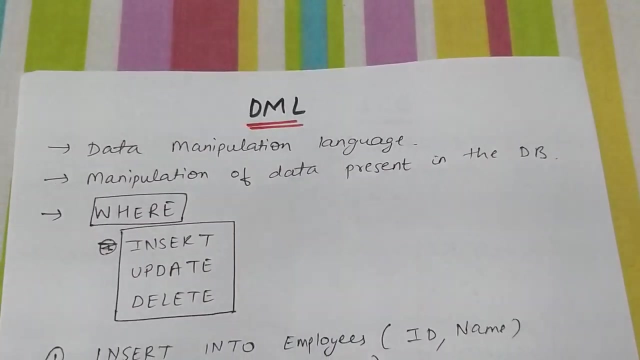 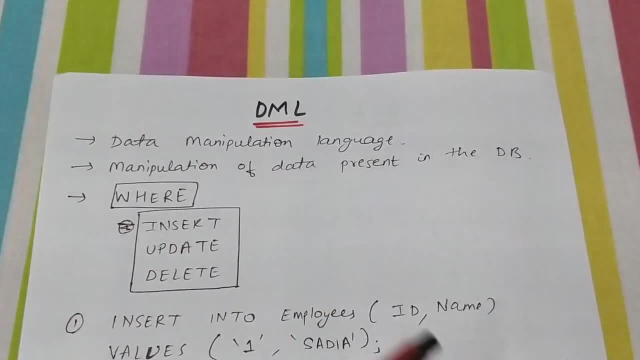 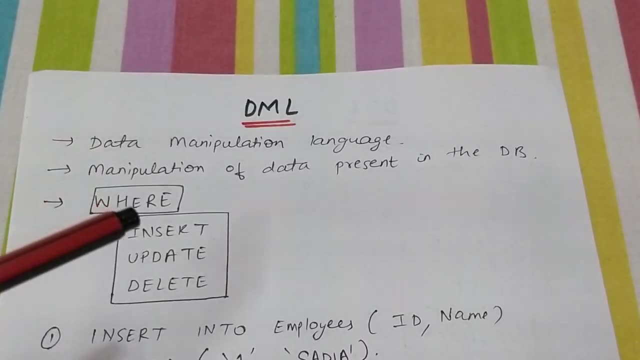 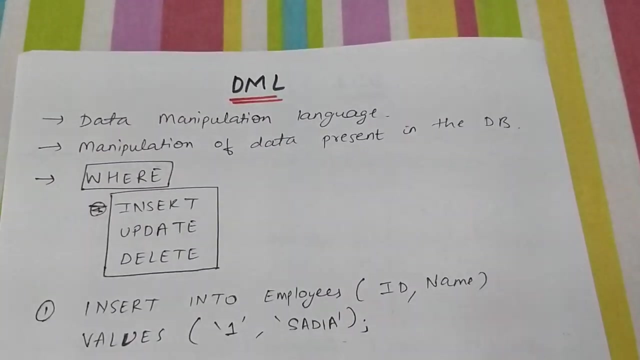 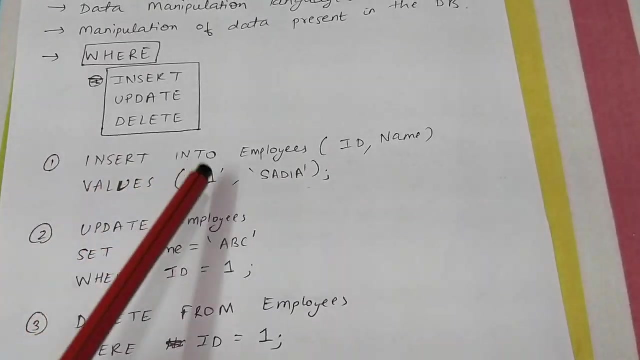 we are going to manipulate it. Basically, we are going to update any value in the row or delete that particular row, or insert a particular row. Okay, so basically we are playing with data over here and hence it is data manipulation language. So there are three commands in it: insert, update and delete. So let's see the three of them. So one is: insert into employees the name of the table. insert into employees whatever column name. 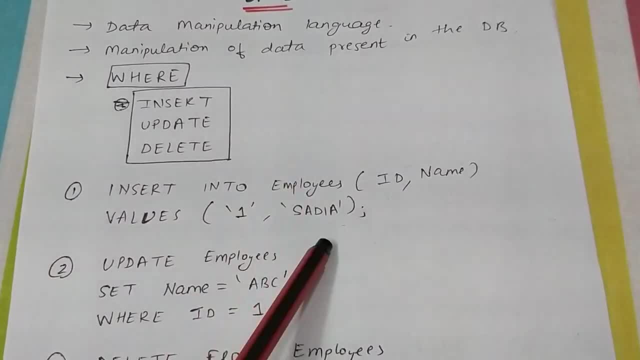 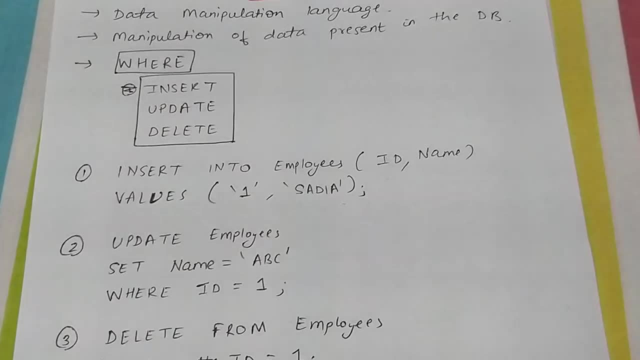 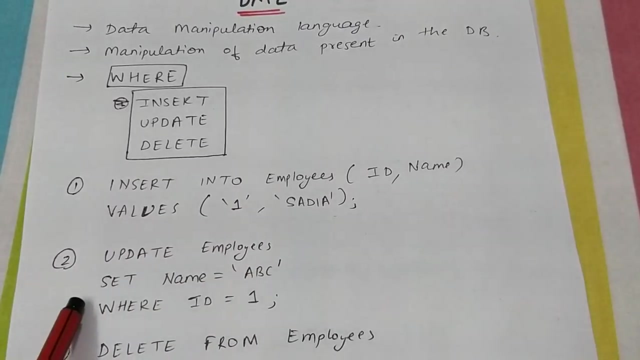 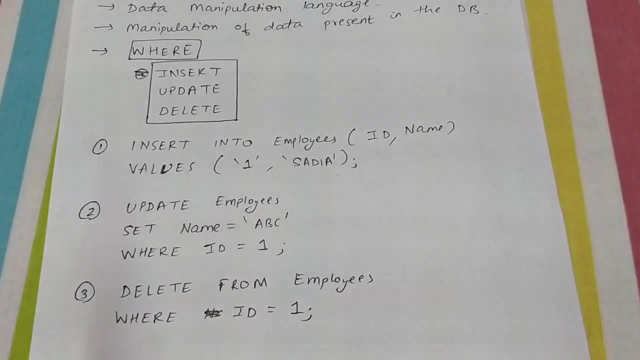 So these are the column names, values and whatever value. you want to insert one and whatever name. And then second one is update. You are updating a value, a value in a particular row. You are changing the value in a particular row, that is update. So update employees that this is the table name. set name is equal to whatever where ID is equal to one. Third is delete command. So here we are deleting a particular delete from employees where ID is equal to one. 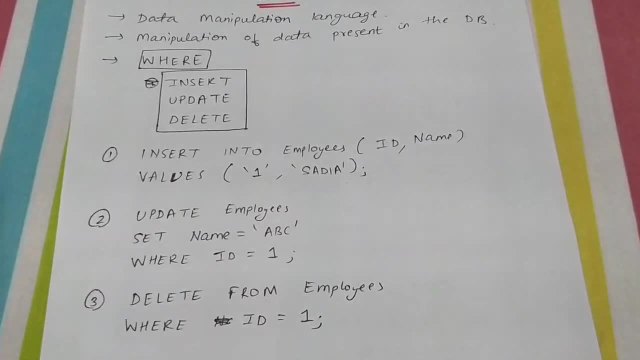 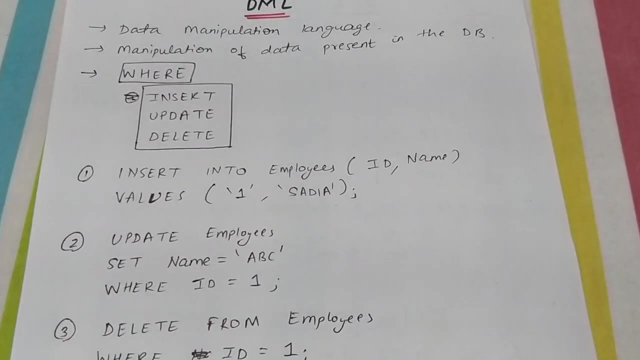 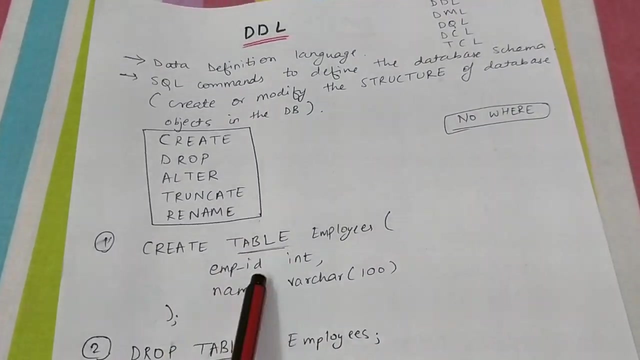 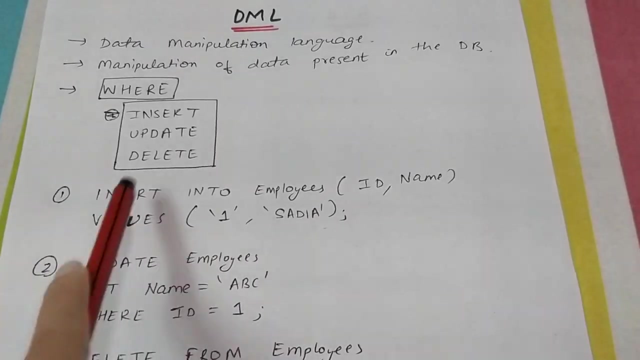 So there are few things which you should remember in DML. So one thing is that you never write the word table, As we used to write in DDL commands like create table this and this or drop table this and this. the word table is used in it, Like this: create table, drop table. But in DML we do not use the word table, Simply we write: insert into employees, update employees, delete from employees, whatever. 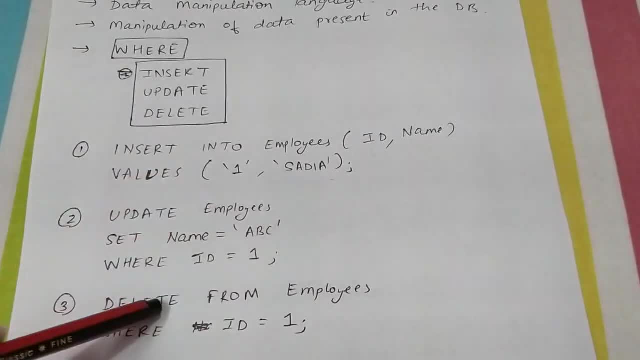 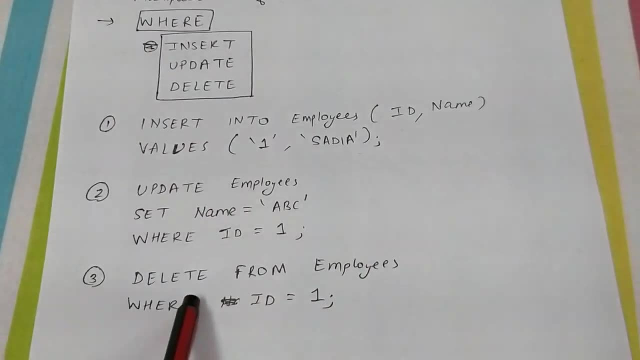 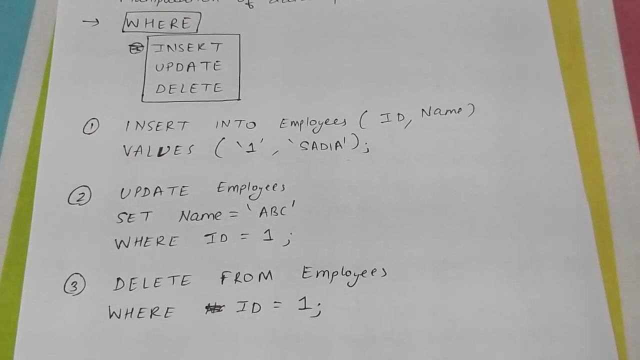 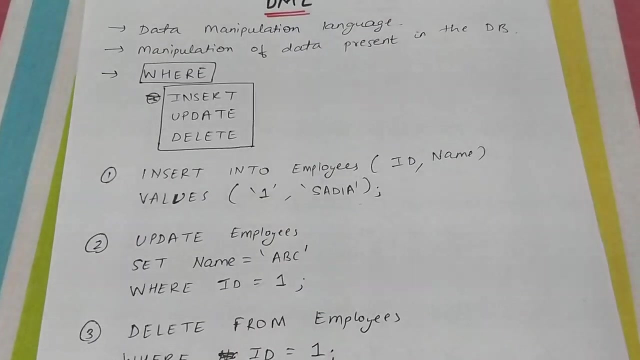 Where in these options, Whereas in DDL you cannot use where. But in these cases we can use where. We cannot use where in insert, but definitely in update and delete we can use where. So this is what DML is: data manipulation language. I hope it is clear. Please do subscribe to the channel for more such videos. Thank you.